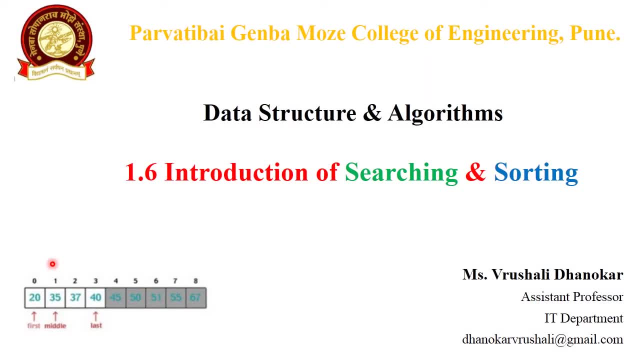 Good morning everyone. I am Rishali Dhanokar, Assistant Professor, IT Department. In my last video, we learned about data structures, then their classification, abstract data types and also arrays and concept of arrays and recursion. Now, in this video, we will learn. 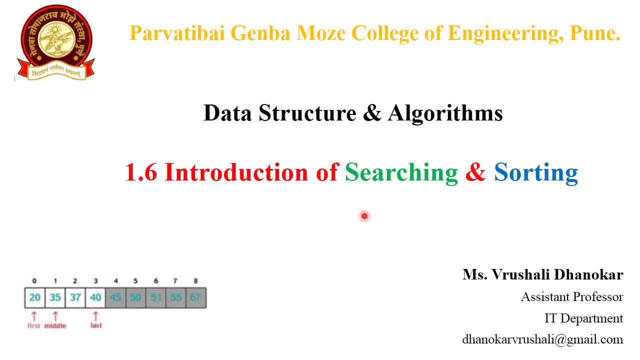 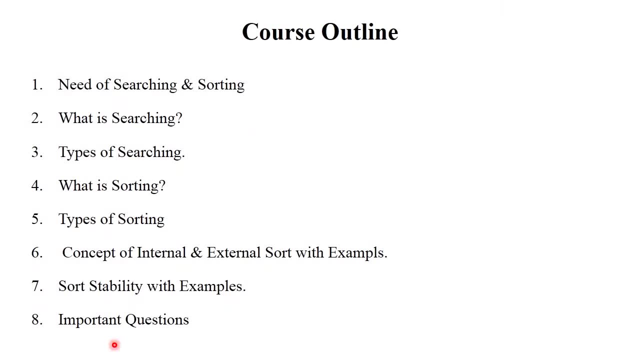 about introduction of searching and sorting. So let's see what is meant by searching and sorting in data structure Next. So following points are covered in this video, which includes need of searching and sorting. about searching and sorting, their types, concept of internal. 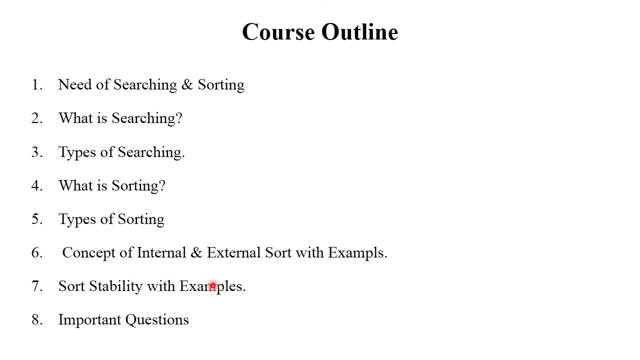 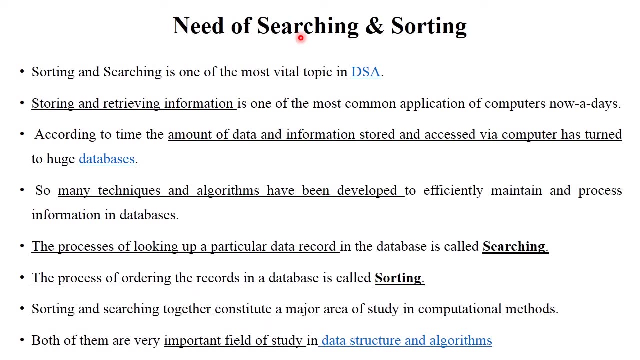 and external sort with examples, sort stability with examples, And also there are some important question which frequently asked in exam. Okay, so let's see need of searching and sorting Next. So, need of searching and sorting. We know that nowadays, large amount of data is available. 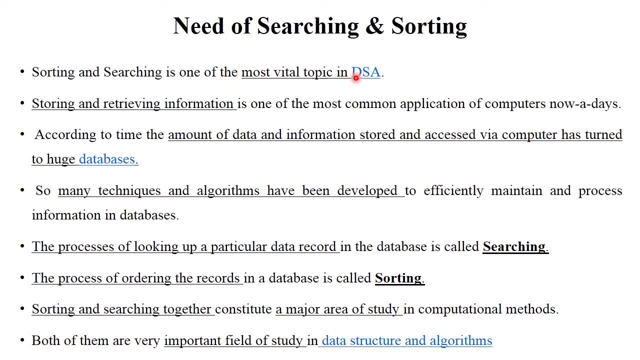 So sorting and searching is one of the most vital topic in data structure and algorithm. Storing and retrieving information is one of the most common application for computer nowadays, According the time, amount of data and information stored and access via computer in huge database right. We use huge number of database and storing and retrieving 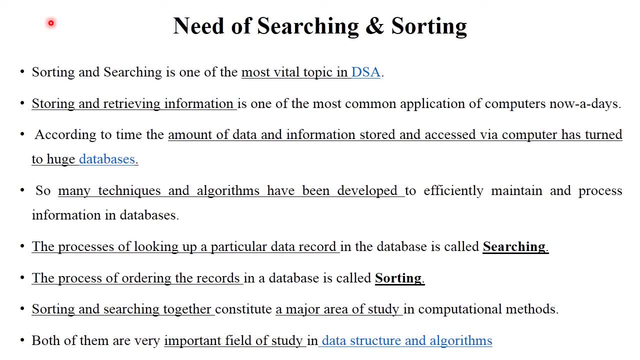 of information is very easy because of searching and sorting concepts Clear Now there are so many techniques and algorithms have been developed efficiently maintain and process the information in database. So, exactly, searching means what? The process of looking up a particular data record, If you want to search a particular data in large number of database, this process 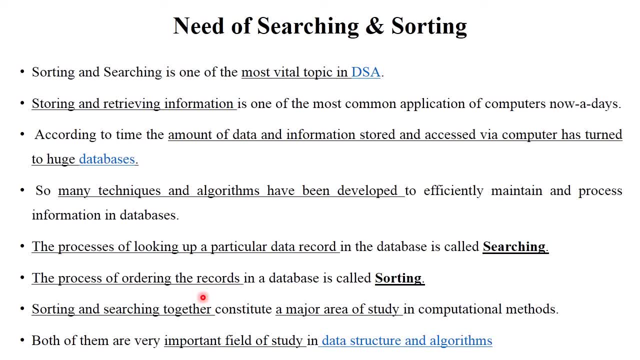 is called as searching, And sorting means the process of ordering of records, Either arrange the order in a large number of database or sort the data in large number of database, Ascending or descending. So this concept is called sorting, Sorting and searching together. 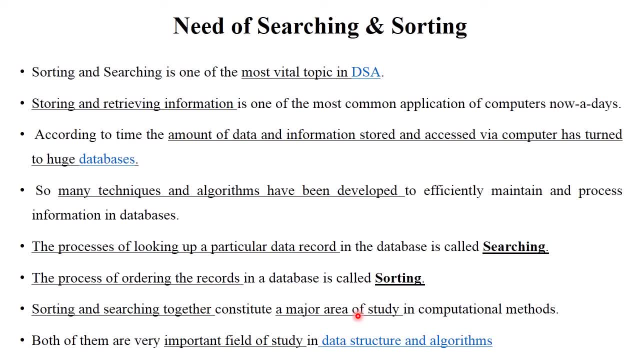 constitute a major area of study in computational methods And both of them are very important field of study in data structure and algorithms. Now, in this part or in this concept, we learn different types of searching techniques, sorting techniques with implementation, Clear Now. 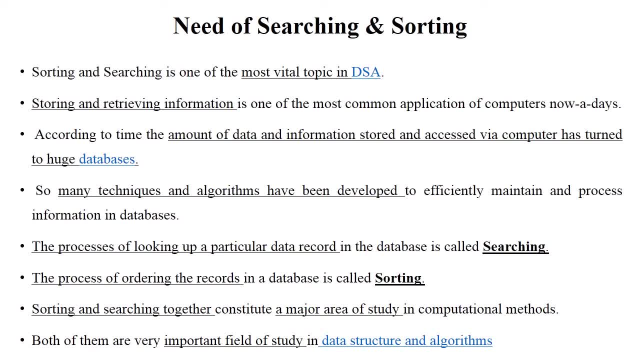 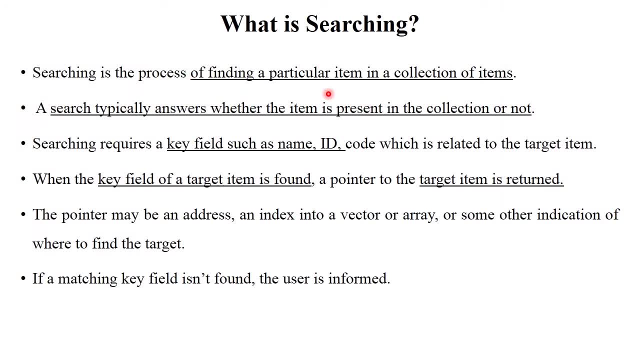 you should understand about need of searching and sorting Next. So first, what is searching in detail Searching is the process of finding the particular item in a collections of item. A search typically answers whether the item is present in the collection or not. If item is present, then they return the search item. If item is not, 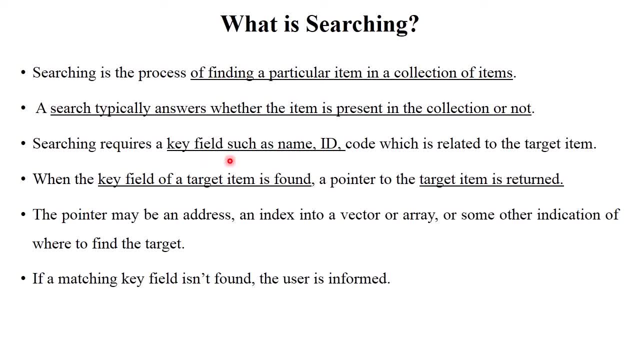 present, then they return the null. Searching requires key field such as name and id, Or we can say it requires unique identity which is related to the target item. If there is student database and available, then it is a search item. If there is student database. 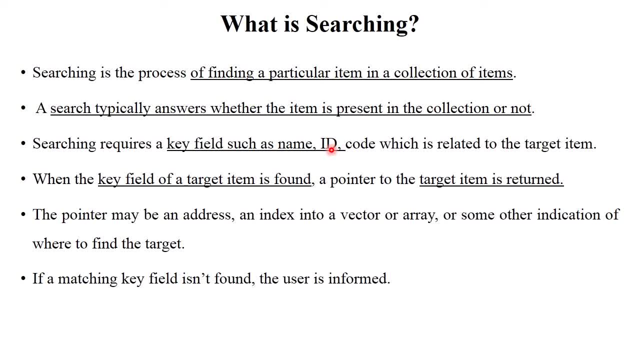 and available, then we want to, or we will, search each and every student according to their role number. So role number is a unique identity Clear. So when the key field of target item is found, the pointer to the target item is returned. Otherwise returns null. 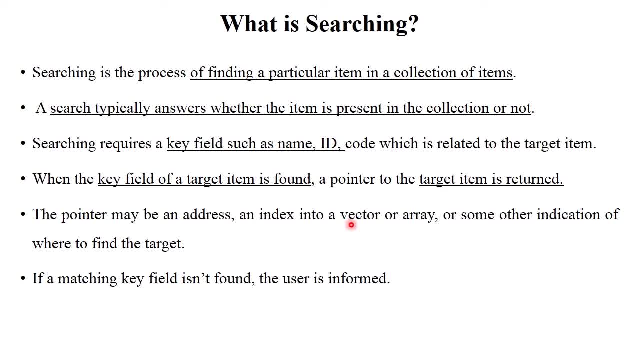 The pointer maybe means address, index, vector or array of that particular searching item. Clear: If matching case found isn't found, then user is informed. If the matching case data is found, then also that particular data is written. or if data is not found, 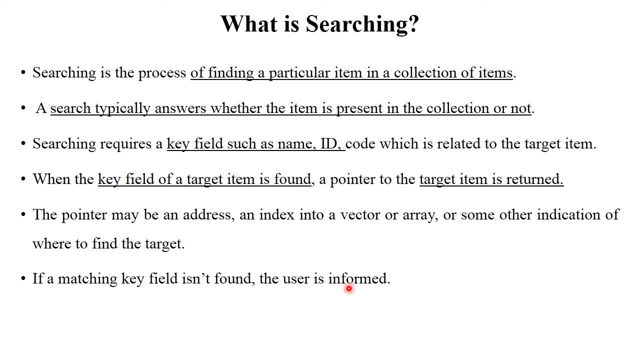 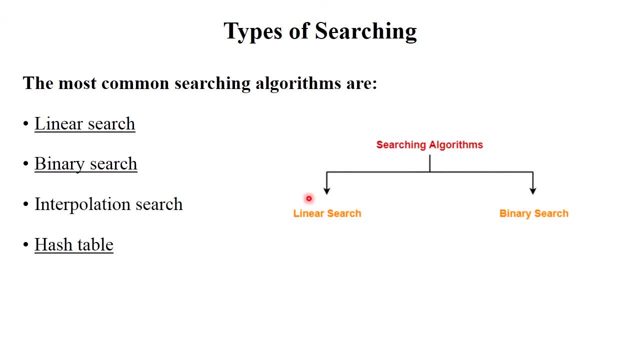 then they return the null value or they inform the user clear. so this is the concept of searching. next, the next types of searching. the most common searching algorithms are linear search, binary search, interpolation search and hash table. inner syllabus included linear binary and hash table. so the main searching algorithms are linear. 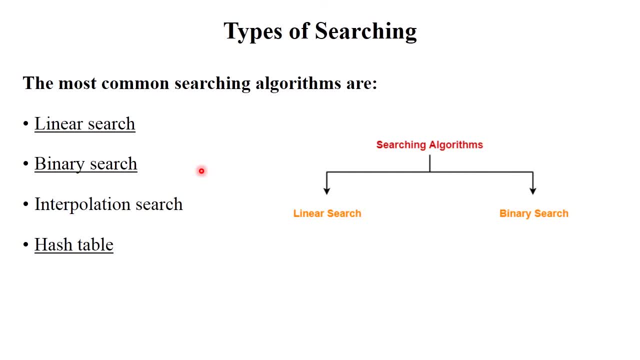 and binary search. in this video I am just explaining about the concept of this searching technique. okay, in my next video I will explain in detail about linear search, binary search, with example and implementation clear. next, what is sorting? sorting is a process of to placing the elements from a 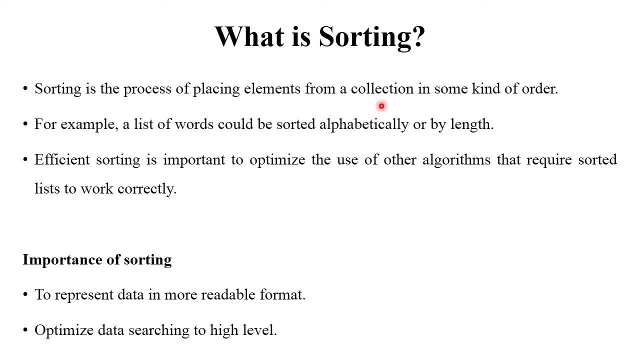 collections of item in proper order, clear. for example, list of words could be sorted alphabetically or by length. so for sorting there are different logics are applied. efficient sorting is an important to optimize the use of other algorithms that require sorted list to work correctly. I will give you one example: in your contact list, in your 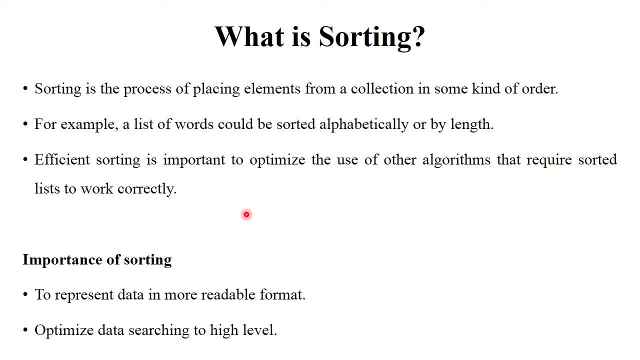 mobile. there is contact list is available and this contact list is already in sorted format from A to Z. why? because access to the list is already in sorted format from A to Z. why? because access- each and every number- is easy to find out and in contact list there is search. 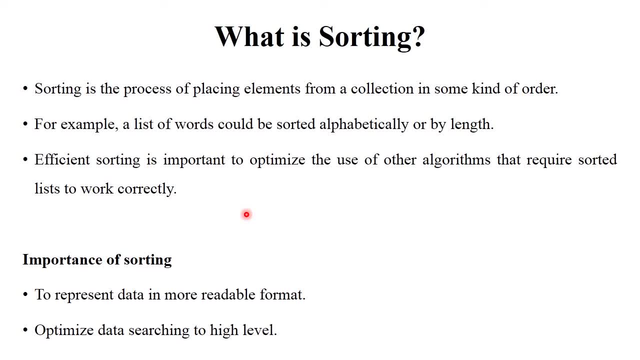 bar is appear according, or you, by using this search bar, you want to search any number in your list. so this is the main example of searching and sorting. so what is the importance of sorting? it represent data in more readable format and also optimize data searching in high level. it can do each and every. 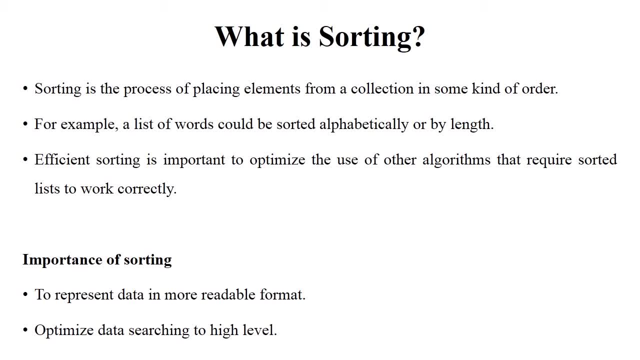 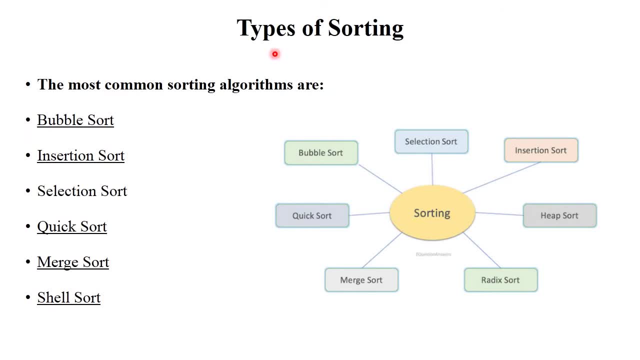 purposes most easiest way and in less time, complexity clear. this is called as sorting. next of the next one is types of sorting. the most common sorting algorithms are bubble sort, insertion sort, selection sort, quick sort, merge sort and shell sort. quick sort is one of the fastest sorting. 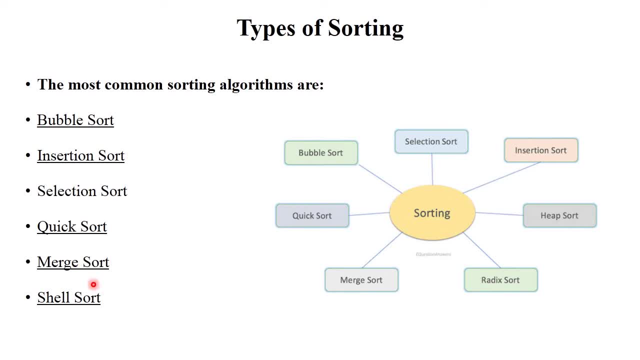 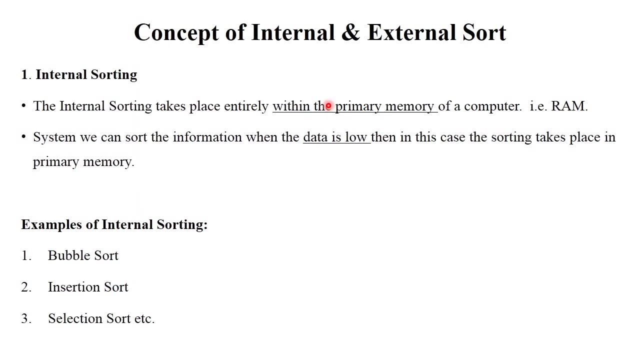 technique. so this: all sorting algorithms are included in your syllabus. I will explain each and every sorting algorithms in my next video with algorithm examples and implementation. ok, next, now again there is concept of internal and external sort. so what is mean by internal sort? the internal represents the internal memory. 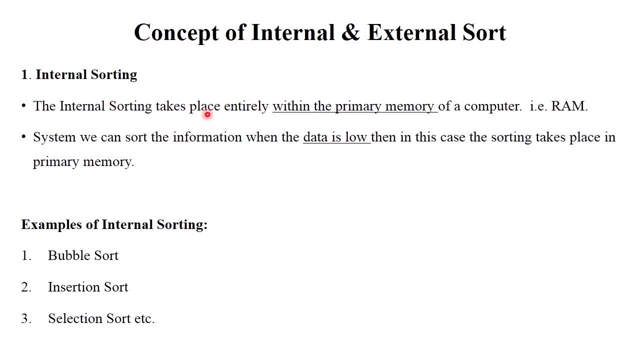 or we can say primary memory. so internal sorting takes place entirely within the primary memory of computer. or primary memory means RAM, that is random access memory for internal sorting. it requires less amount of data. it works only on less amount of data or in this case, sorting takes place in primary. 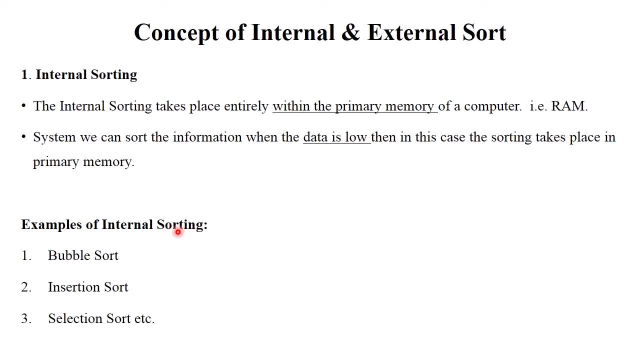 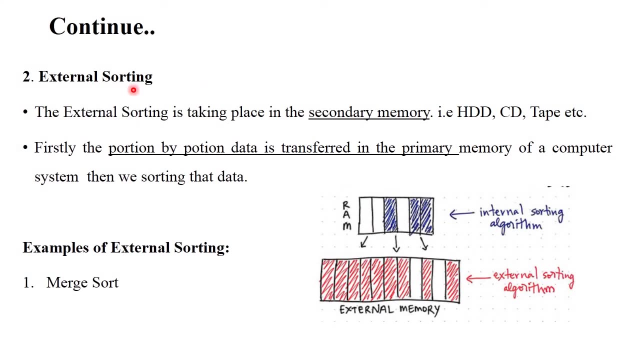 memory. the examples of internal sorting are like bubble sort, insertion sort, selection, sort, etc. this all sorting algorithms are work on low amount of data, clear next. the next one is external sorting. so external sorting is completely opposite of internal sorting. external sorting is taking place on the secondary 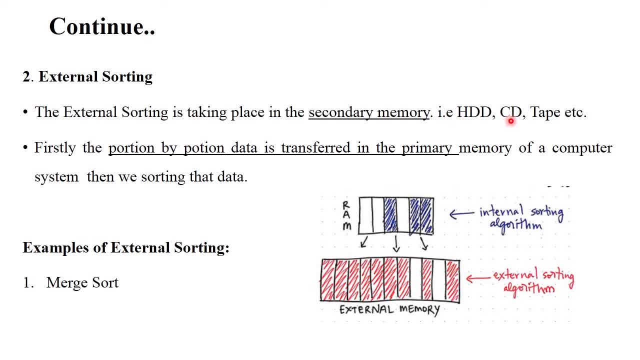 memory. Secondary memory means HDD, CD Tab, etc. The first portion by portion data is transferred into the primary memory of computer. then we sorting the data In external sorting. all the data is stored in external memory. Clear, that is secondary memory. and after sorting, 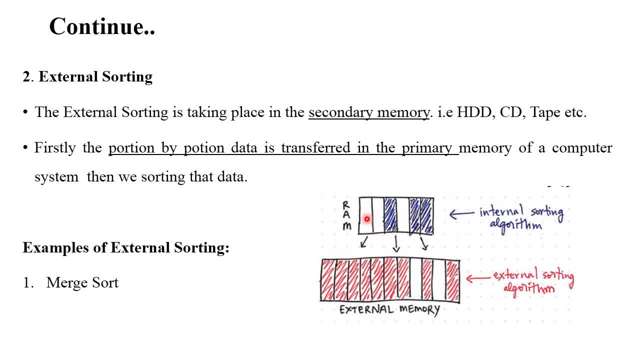 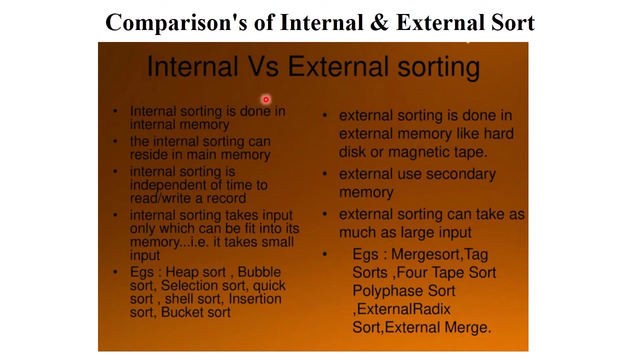 this data will be stored in internal memory, that is, RAM. The example of external sorting is merge-sort. Merge sort, quick sort. this type of algorithm, sorting algorithm, will be used for large amount of data. So this is the concept of internal and external sorting. next see: here there is a difference between internal vs external sorting. Internal sorting: 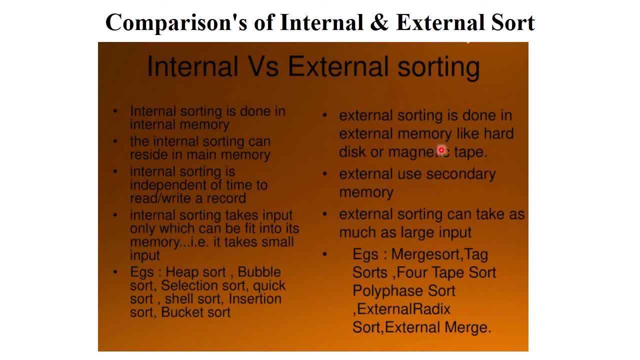 done in internal memory, external sorting done in external memory like HDD, Tab etc. Internal sorting can resides in main memory and external sorting coners can resides only external memory. as we know, in hard disk type tv lidar Internal is used secondary memory for large amount of data storage purpose. 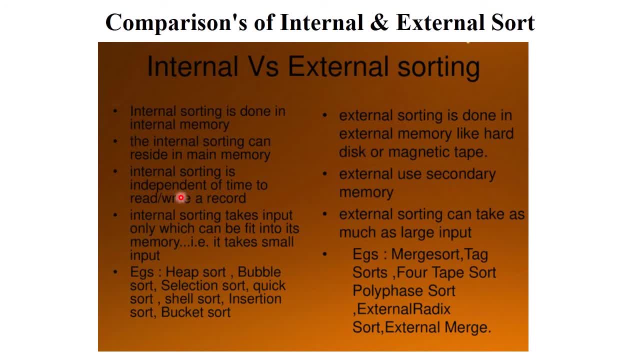 Clear. Internal sorting is independent of time to read and write record. Internal sorting also takes input which can be fit into its memory. It takes small input. Okay, Only required data. The size of primary memory is only required for internal sorting amount. 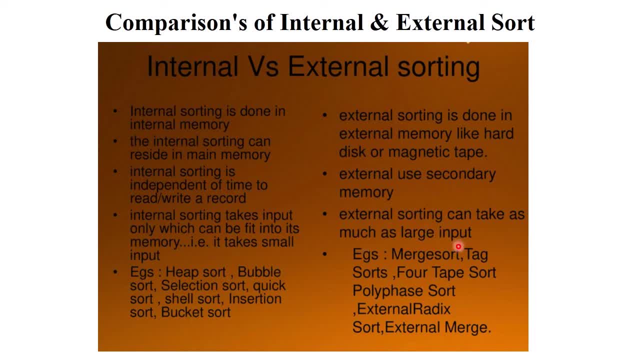 But in external sorting it use primary memory as well as secondary memory storage because data is in large format, Clear. The example of internal sorting are bubble sort, selection, quick sort, insertion, bucket sort, heap sort, etc. And examples of external sorting are merge sort and also there are some radix sort, polyphase. 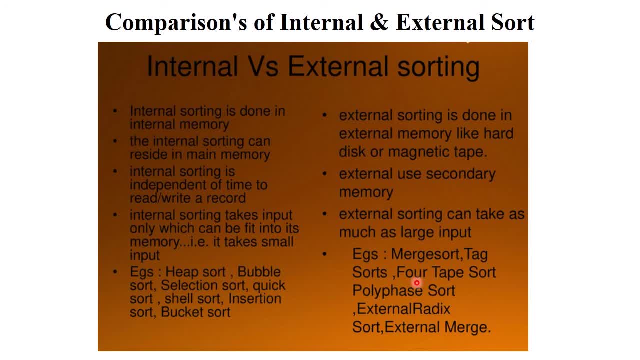 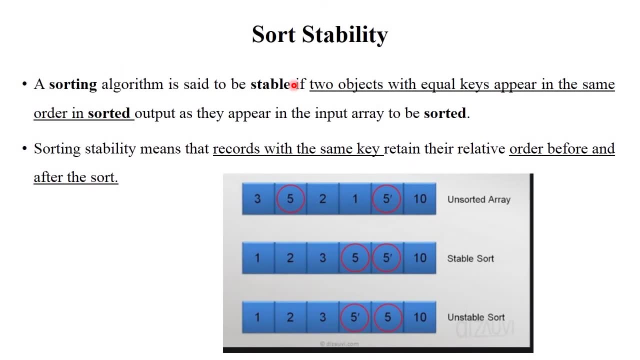 sort, etc. So we will see in detail each and every sorting algorithms in my next video, Clear Next. Now again, there is one concept like sort stability. So this word stable, Stable means constant, Right. So what is mean by sort stability? 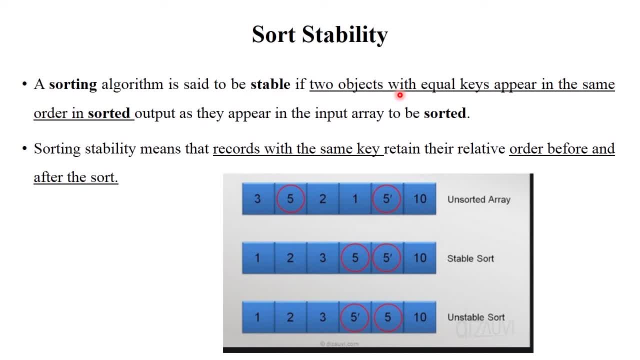 The sorting algorithm is said to be stable if two objects with equal key appears in the same order in sorted. Now see here In this diagram: unsorted array is 3, 5, 2, 1, 5, 10.. 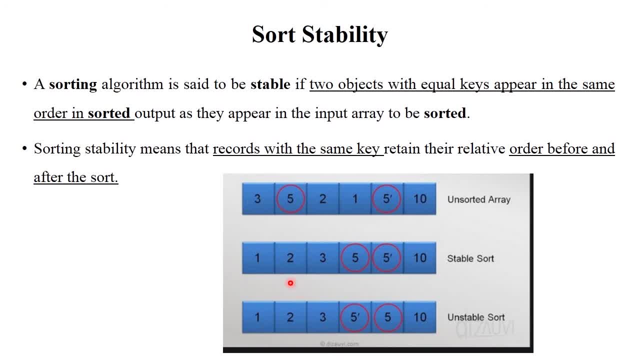 Okay, Then you need to sort this data. After sorting 1,, 2,, 3,, 5,, then 5' and 10.. Now see here The place of 5' and 10.. Okay, 5', and after sorting, the place of 5' is same.